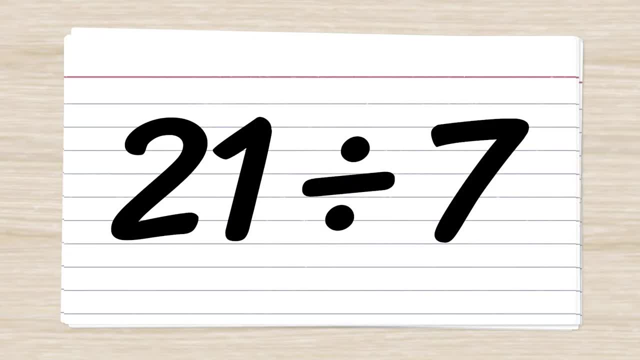 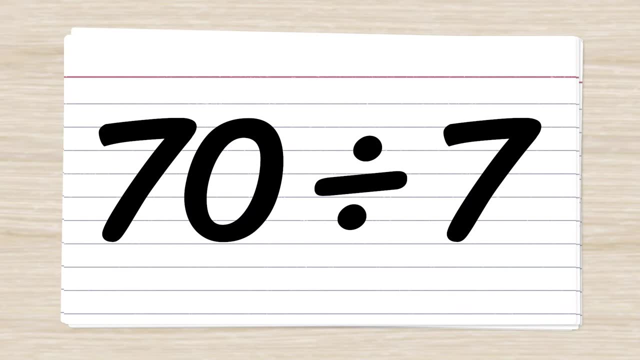 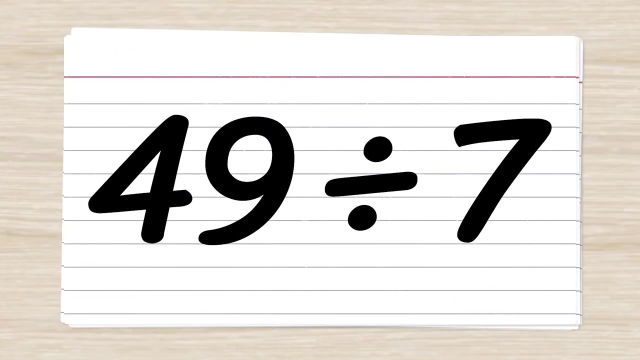 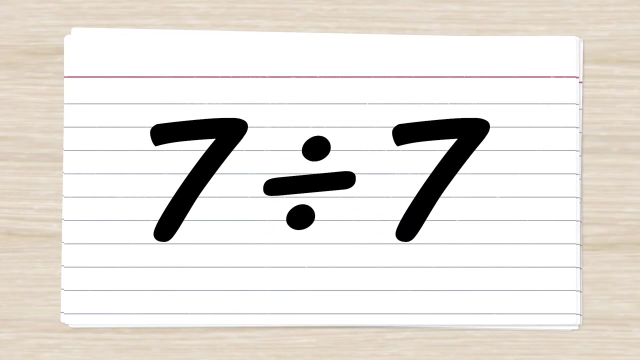 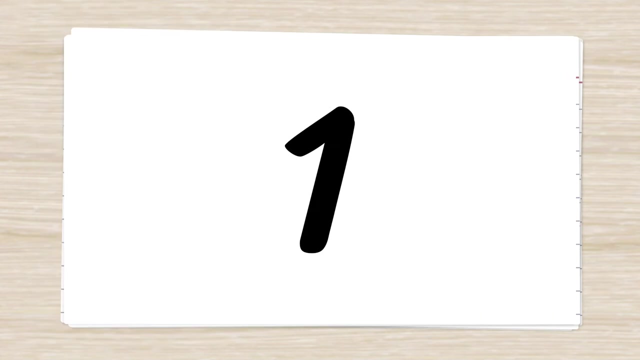 Twenty-one divided by seven. Three Seventy divided by seven. Ten Fifty-six divided by seven. Eight Forty-nine divided by seven. Seven. Seven divided by seven. One Thirty-five divided by seven. Five Sixty-three divided by seven. Nine. 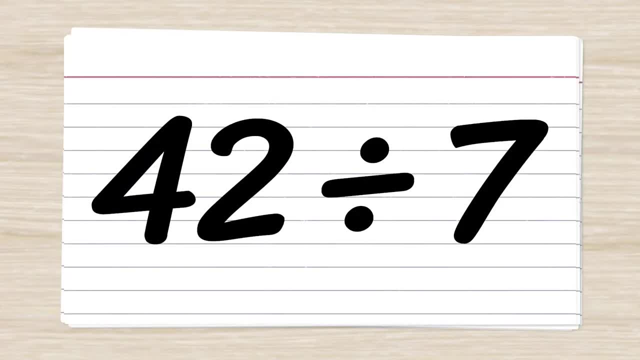 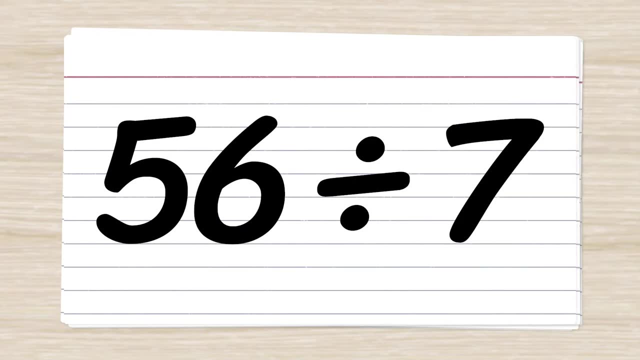 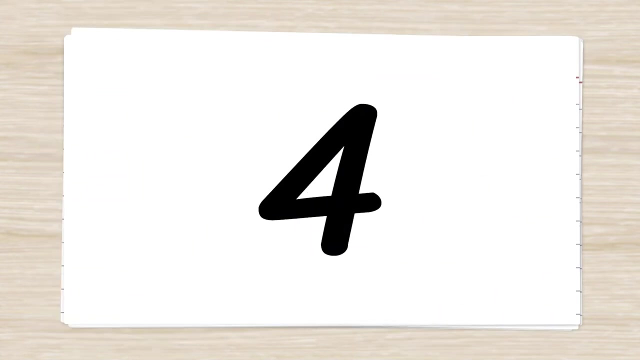 Forty-two divided by seven. Nine. Forty-two divided by seven. Seven, Six, Fifty-six divided by seven. Eight, Twenty-eight divided by seven. Four Twenty-one divided by seven. Three Fourteen divided by seven, Seven, Two. 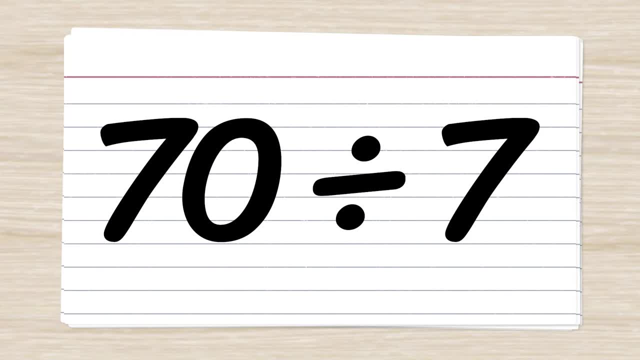 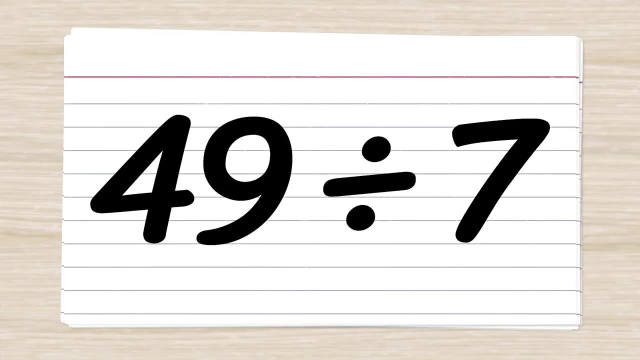 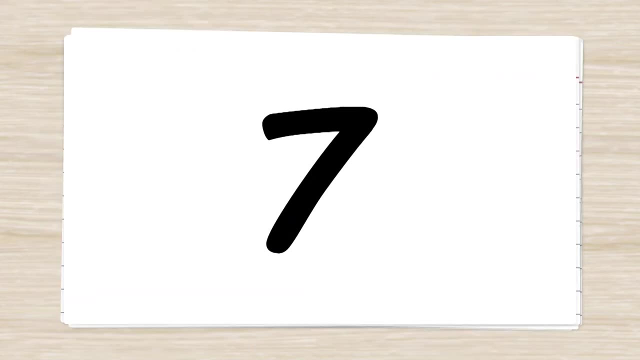 Two, Seventy divided by seven. Seventy divided by seven. Ten, Ten Forty-nine divided by seven. Forty-nine divided by seven. Seven, Seven divided by seven. Seven, Seven divided by seven. Seven. Seven divided by seven, Seven. 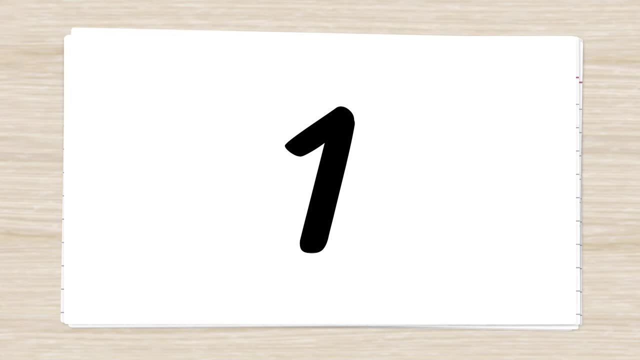 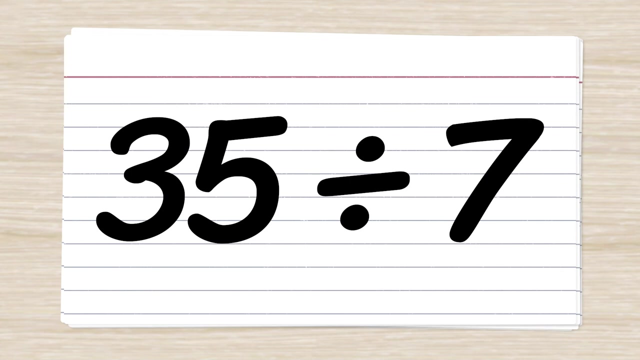 One, One One Twenty-two divided by seven. Seven, Three, Four, Thirty-two divided by seven. Seven, One, One, One, One One One One. Full count tt. Five, Two, Seven, Ten, Fifty-six divided by seven. 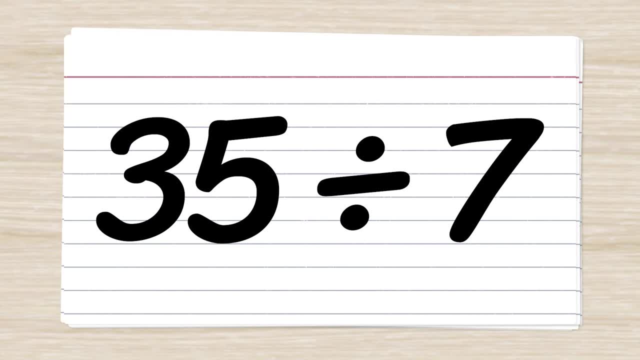 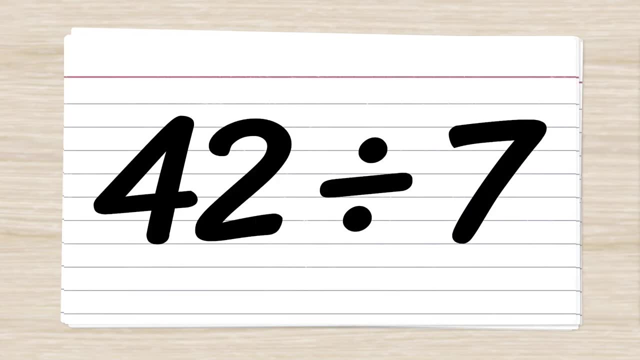 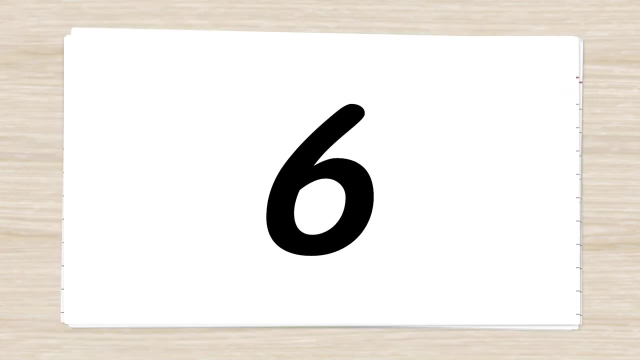 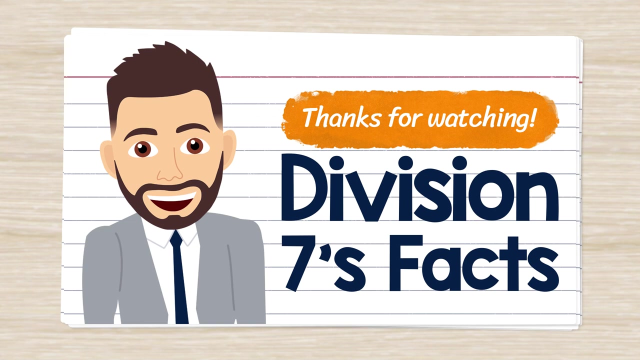 Eight, Thirty-five divided by seven, Five, Forty-two divided by seven, Six, Twenty-eight divided by seven: Four. And that's it for the flashcards in this video. Thanks so much for watching. Until next time, peace. 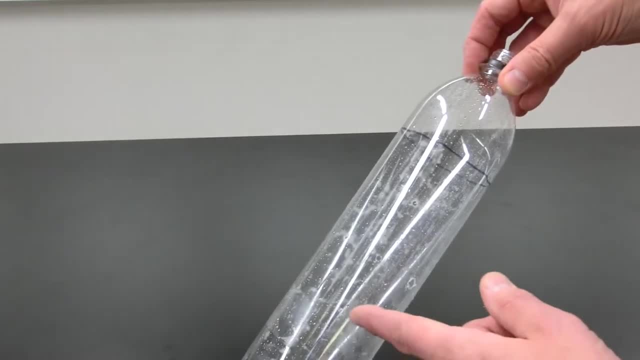 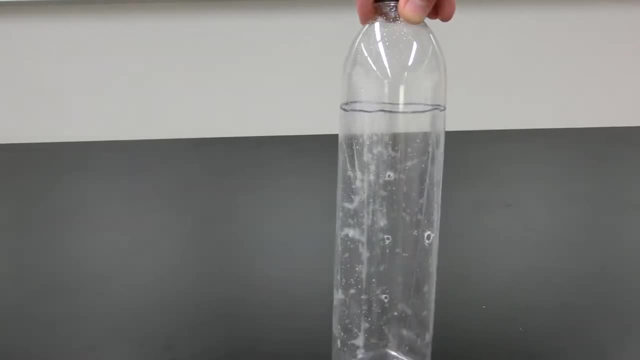 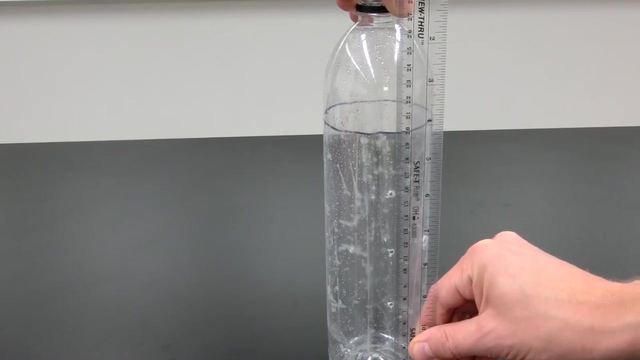 In this experiment you'll study fluid dynamics using a plastic bottle full of water. The bottle has three holes of the same size and three holes at the same height but different sizes. Bernoulli's Principle says that the flow velocity of water out of each hole should be determined only by the distance of each hole below the water level. 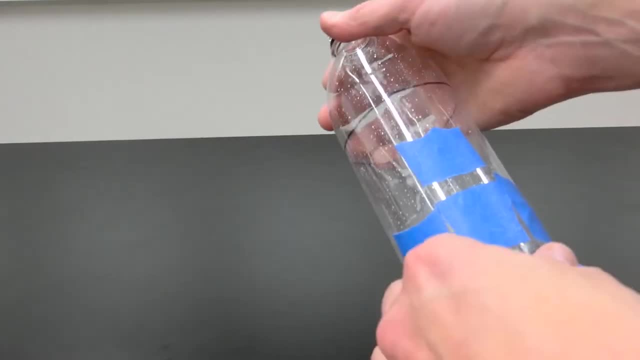 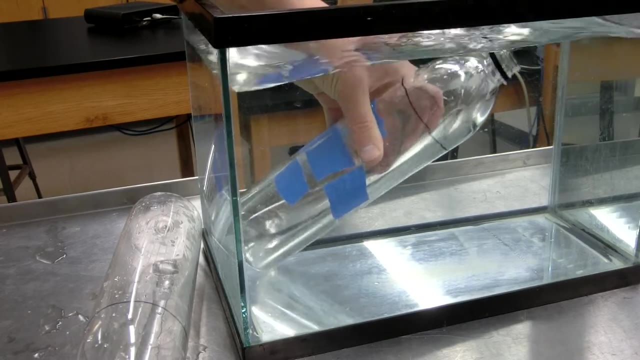 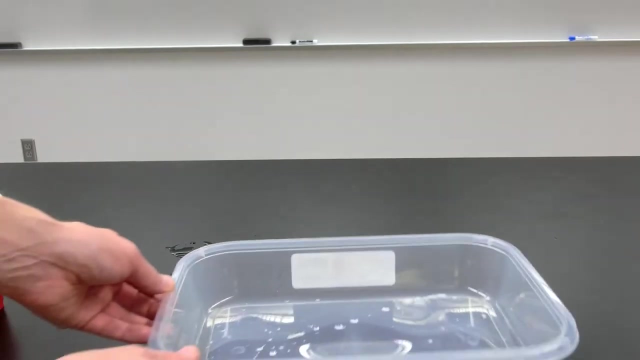 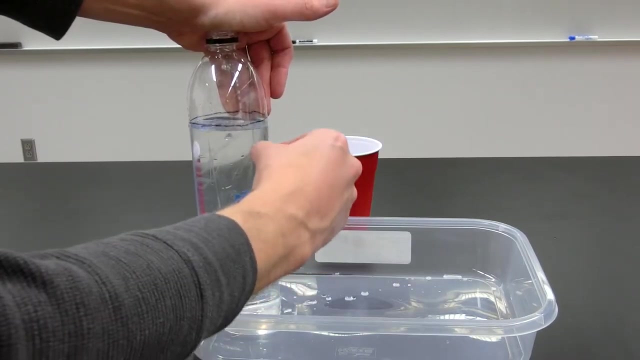 Use some tape to cover up the holes in the bottle. Fill your bottle with water up to the fill line. You can use the bottle's cap or hold your hand over the top to prevent water from spilling out when you remove a piece of tape. 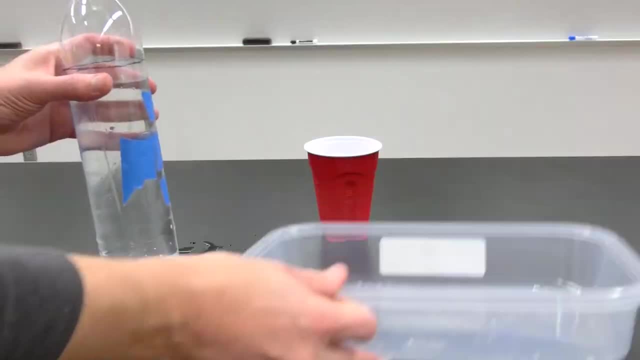 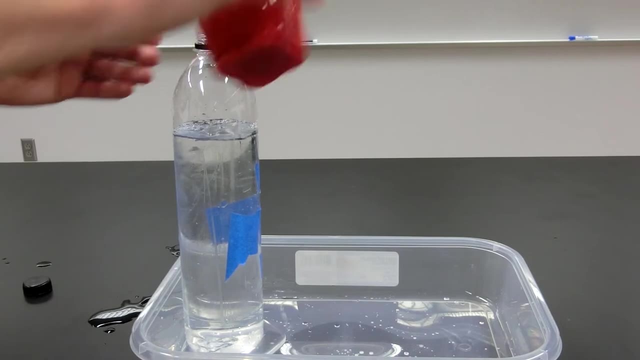 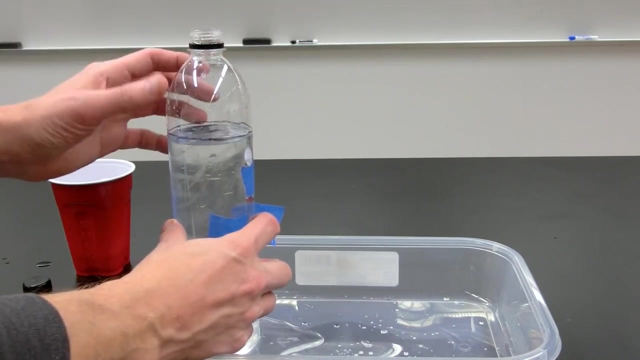 Remember to add water back up to the fill line before removing each piece of tape to see how far the water stream travels. Remember to add water back up to the fill line before removing each piece of tape to see how far the water stream travels. Remember to add water back up to the fill line before removing each piece of tape to see how far the water stream travels. 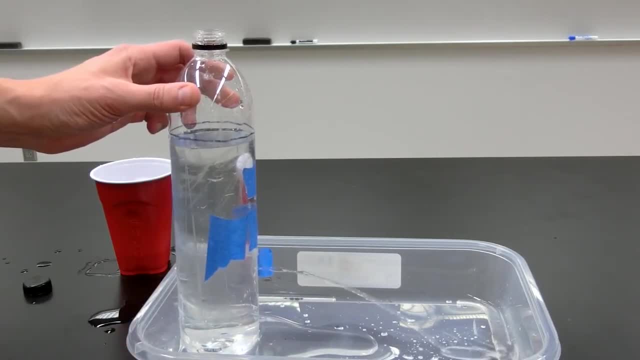